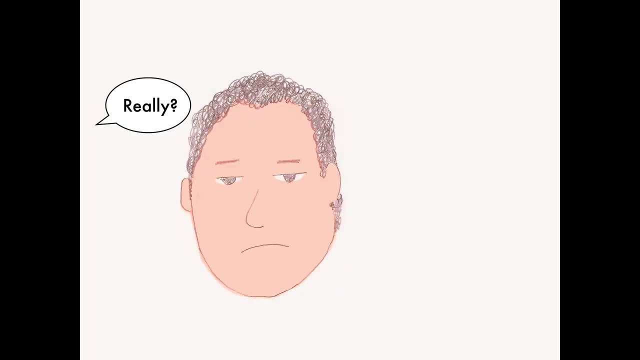 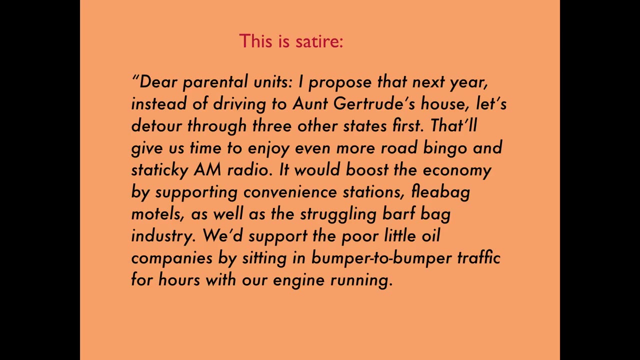 common. Well, that's just sarcasm, and most teenagers know all about sarcasm. But if you were to write a letter to your parents, dear parental units, I propose that next year, instead of driving to Aunt Gertrude's house, let's detour through three other states. 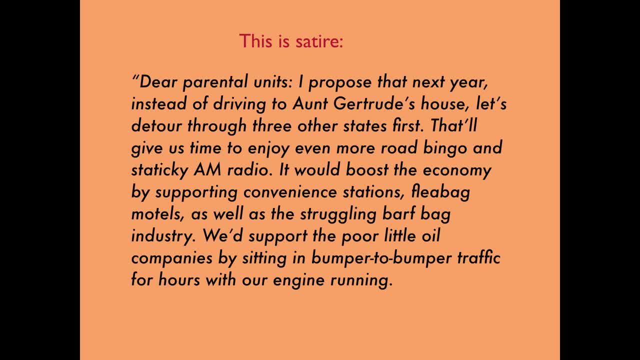 first. That'll give us time to enjoy even more road bingo and staticky AM radio. It would boost the economy by supporting convenience stations, fleabag motels, as well as the struggling barf bag industry. We'd support the poor little oil companies by sitting in bumper-to-bumper traffic. 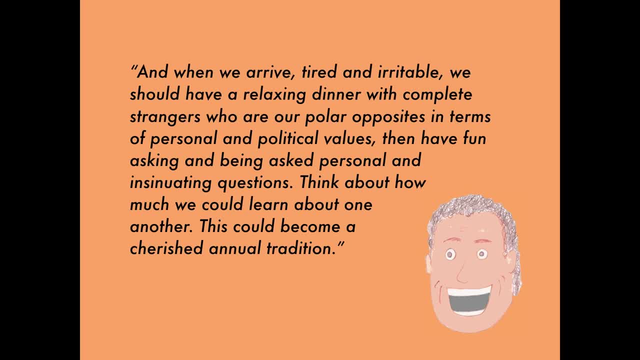 for hours with our engine running And when we arrive tired and irritable. we should have a relaxing dinner with complete strangers Who are our polar opposites in terms of personal and political values. Then have fun asking and being asked personal and insinuating questions. Think about how much we could. 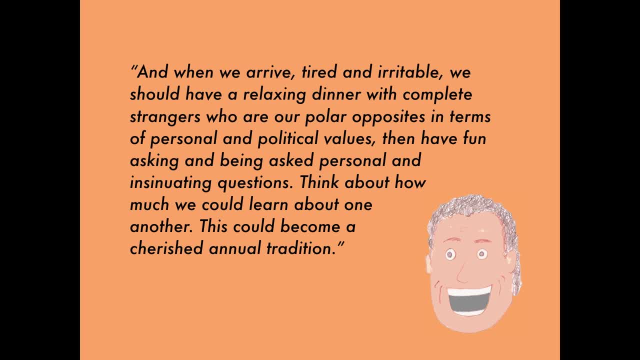 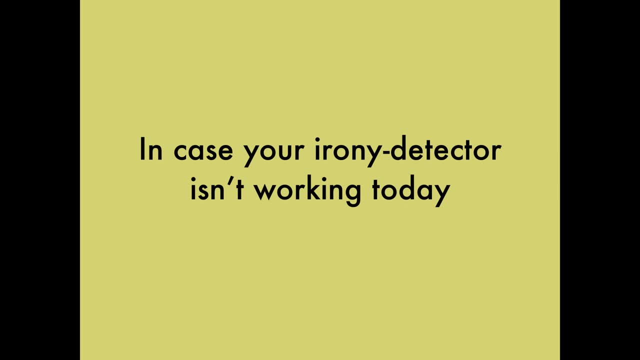 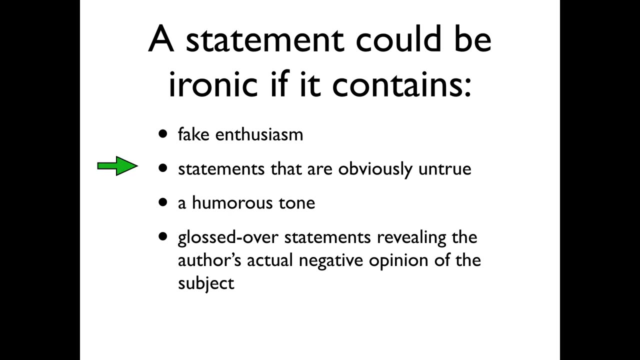 learn about one another. This could become a cherished annual tradition. Well, that would be satire. How can you tell the author is being ironic? A couple of things. First there's the fake enthusiasm. Then there are statements that your reader knows are the opposite of the truth. 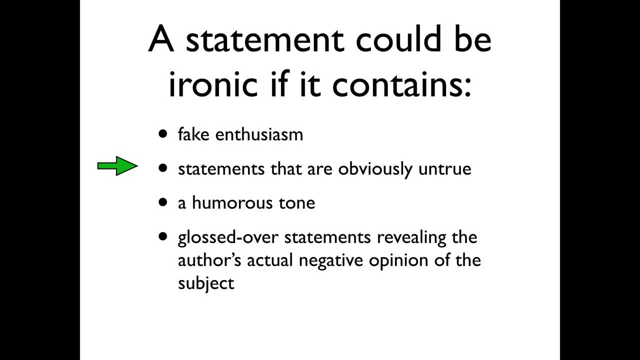 like wanting to play more road bingo And listen to more staticky radio. like describing the ginormous multi-billion dollar oil companies as poor and little. There's a little attempted humor with a barf bag reference, And then there are a few slipped-in statements that reveal how you actually feel like 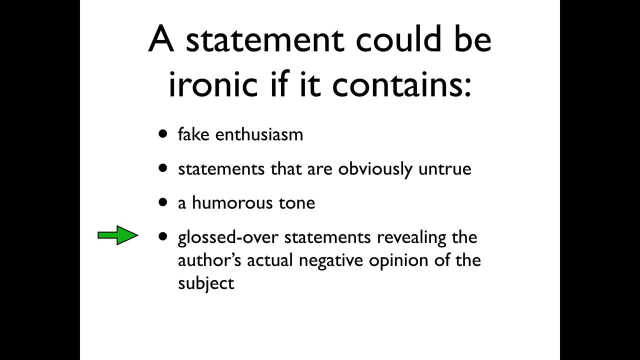 fleabag motels, bumper-to-bumper traffic and strangers who are our polar opposites in terms of our values. So reading this, an alert reader understands. you mean the exact opposite of what you're saying. When you say it's good, you're saying it's bad. When you say it's bad, you're. 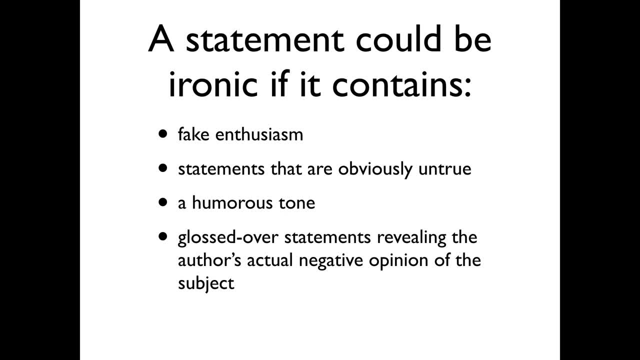 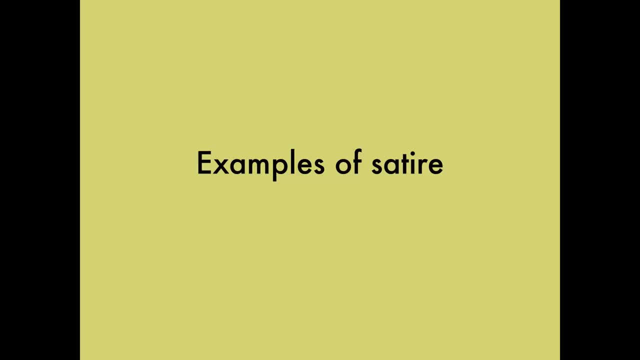 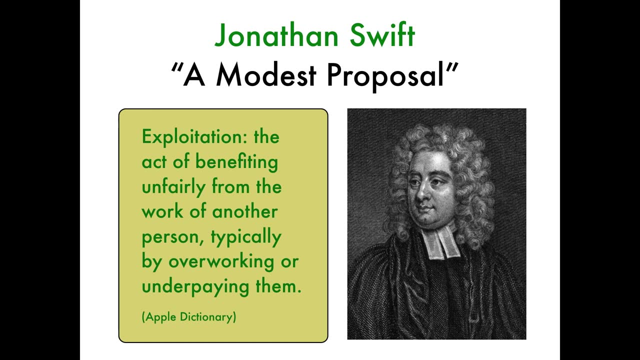 saying it's good that strangers ask you personal questions, You're actually saying you hate it when your second cousin asks: why do you dress like that? A very famous example of satire is Jonathan Swift's A Modest Proposal in which Swift harshly criticizes selfish and exploitative attitudes. 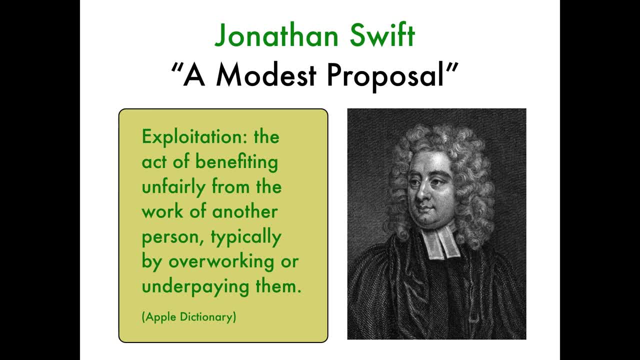 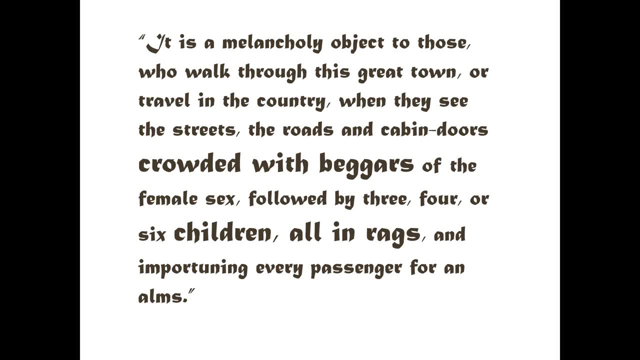 of wealthy Englishmen towards the starving people of Ireland, And they were literally starving to death back then in 1729.. Jonathan Swift first describes the pitiful plight of the poor Irish people in lines like these. Next he proposes a solution: Impoverished Irish mothers can sell their babies to wealthy English. 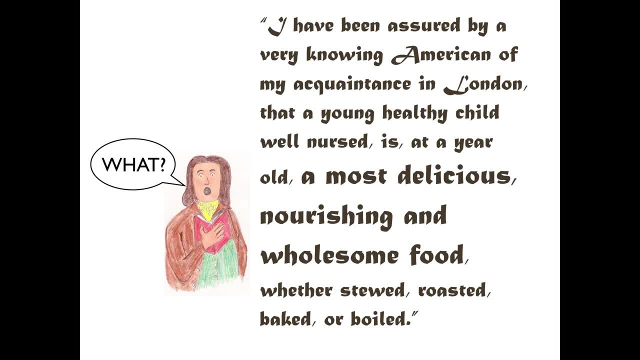 people to be killed and eaten. The Irish parents make a profit and the English get to enjoy- quote- a most delicious, nourishing and wholesome food. After all, their landlords have already figuratively devoured many of these babies' parents. He goes on to explain the many 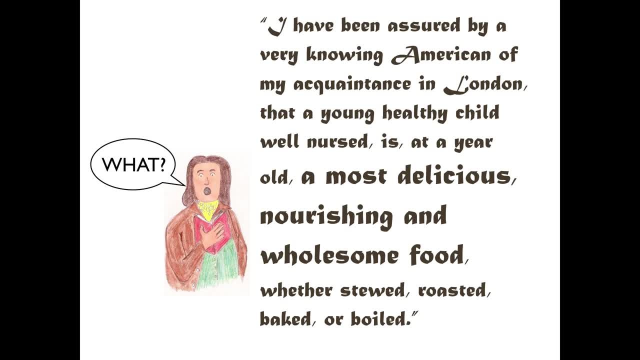 five-year-old Irish mothers who have been killed and eaten. And he says, quote: And this is proposed- with a completely straight face. Naturally his English readers were shocked but when they got Swift's sick joke, most readers could see how the way their fellow 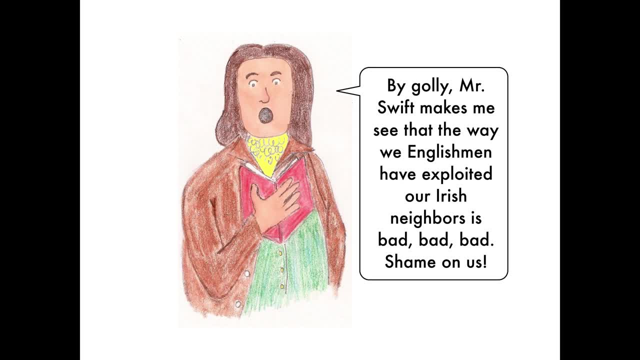 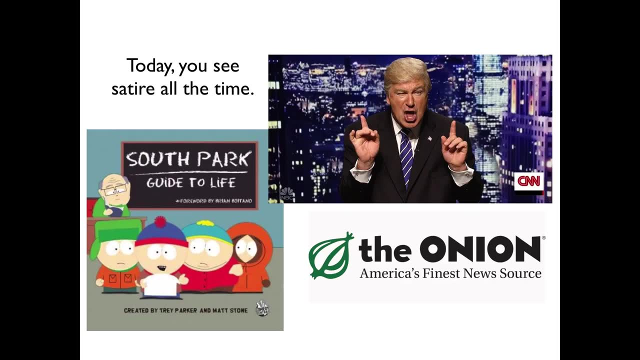 Englishmen were exploiting their neighbors in Ireland was well, not as bad as cannibalizing babies, but it was pretty close. And that's the power of satire. Nowadays you see satire all the time. More recent and lighthearted forms of satire can be seen on. 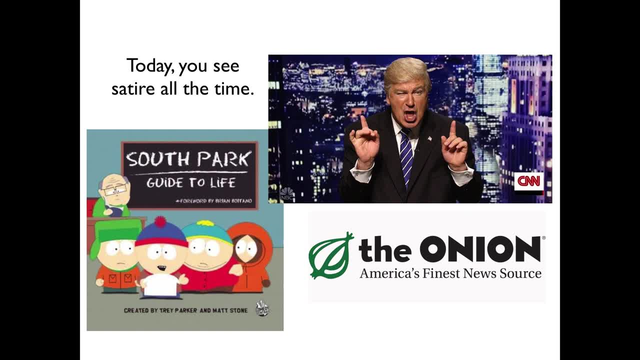 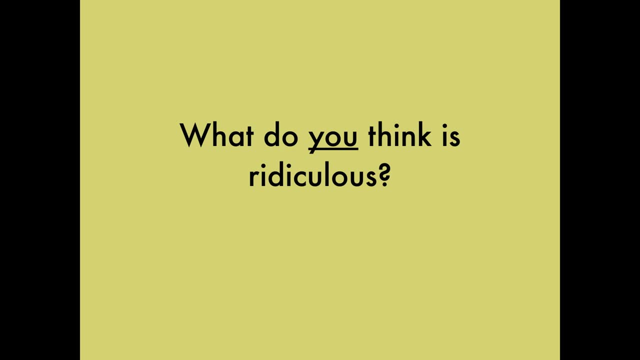 The Onion and South Park. When a TV comedian pretends to be the president and exaggerates the ridiculous things the president says and does, well, that's political satire. So the first thing to do is to think of something you think is ridiculous, Even the nicest person. 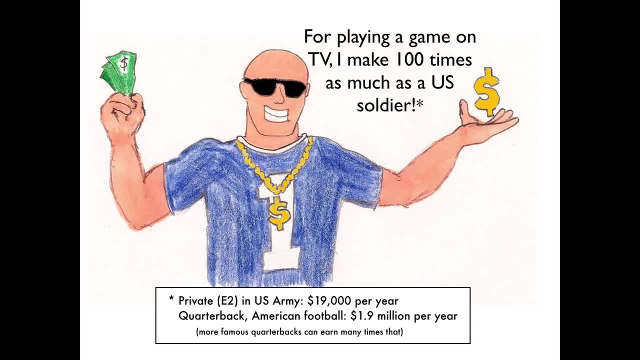 thinks something deserves to be held up to ridicule and scorn. Think Celebrities, professional athletes who make gobs of money, award shows, reality TV, personal electronics, political campaigns, cigarette smoking, YouTube, the state of schools today, people's screwed-up values, fanatical fans of teen pop idols or fanatics of any kind. 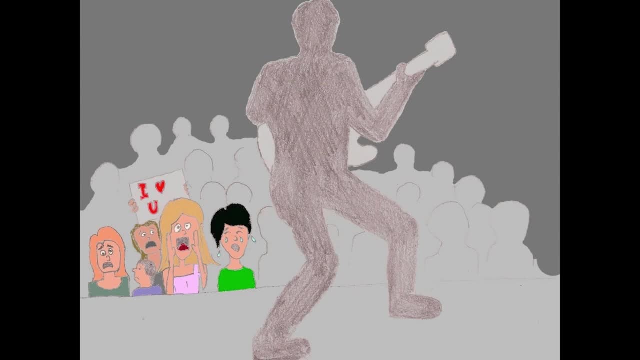 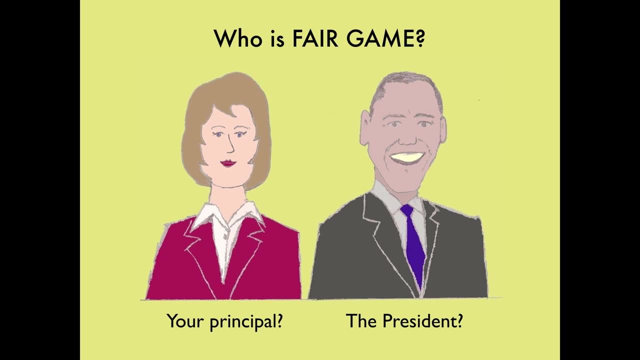 Any of these could be a good subject And, yes, satire can be a little mean, so I'm going to ask you not to write about any particular individual you know personally. That rules out your classmates, your principal, your little brother or sister, But public figures. 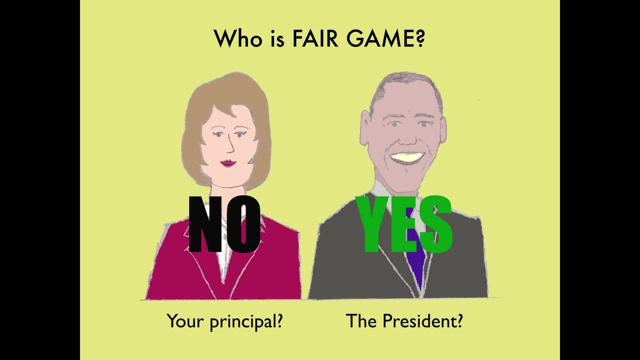 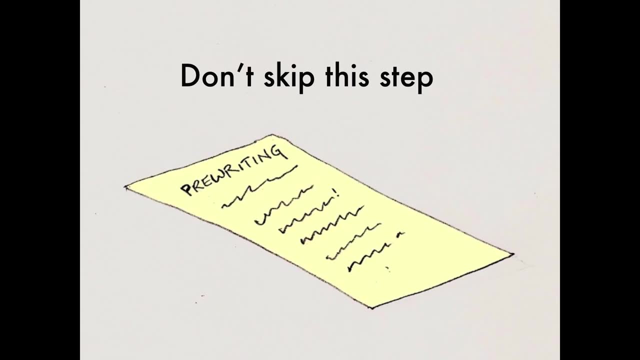 like celebrities or elected officials, are fair game. Once you've picked your subject, you need to make a list of the reasons that person, thing or idea is ridiculous. You need more than one reason. 200 words isn't very long, just about two or three paragraphs. but that doesn't mean you. 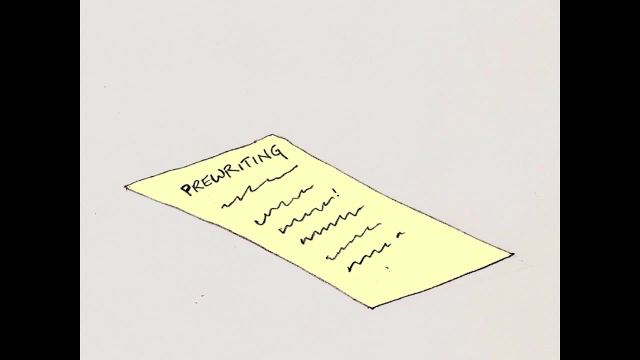 can fill 200 words just saying the same thing over and over. So make a list. After you have your list, write 200 words praising your subject satirically, which means describing your subject in a satirical way. If you have a list, write 200 words praising your subject.